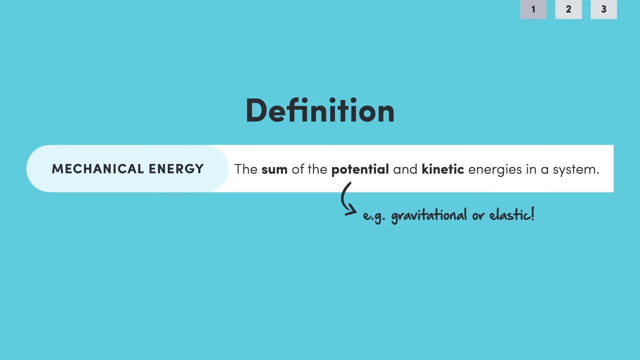 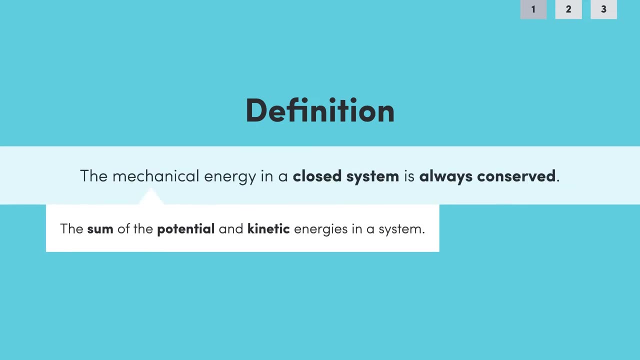 or elastic. However, for this video we'll just be looking at the gravitational potential energy. So the key concept we need to understand in this lesson is that, just like the law of conservation of energy says, the mechanical energy in a closed system is always conserved. 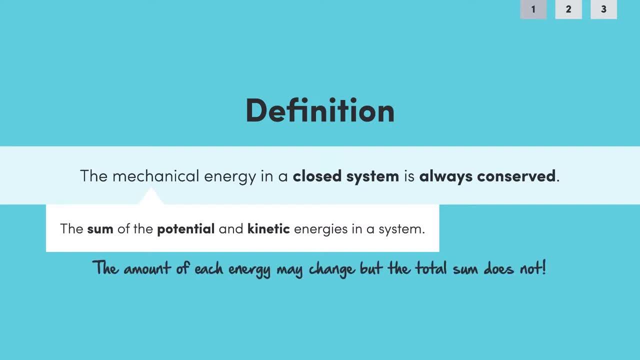 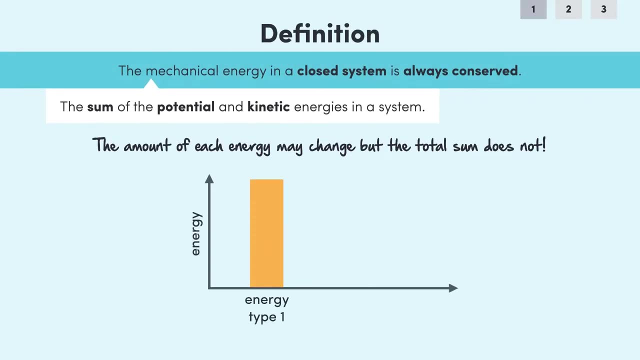 This means that even though the kinetic energy might change and the potential energy might change, the total sum of these two don't change. That is, energy simply transforms from one type to the other. If one goes up, the other goes down. This idea lets us solve a bunch of problems. 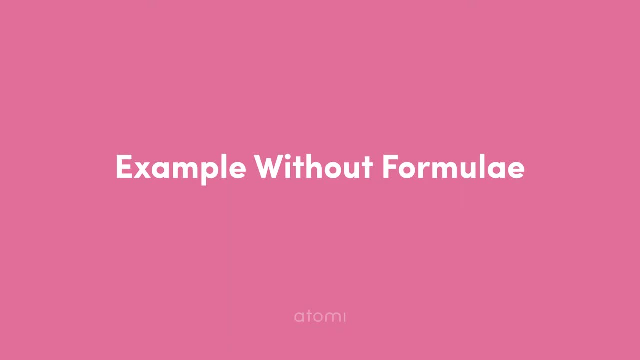 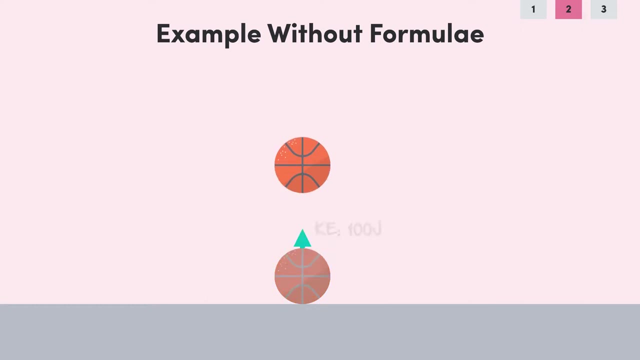 So let's run through an example without formulas, just to get comfortable with this new idea. So let's say we have a ball that starts on the ground. We then launch it into the air by giving it 100 joules of kinetic energy. 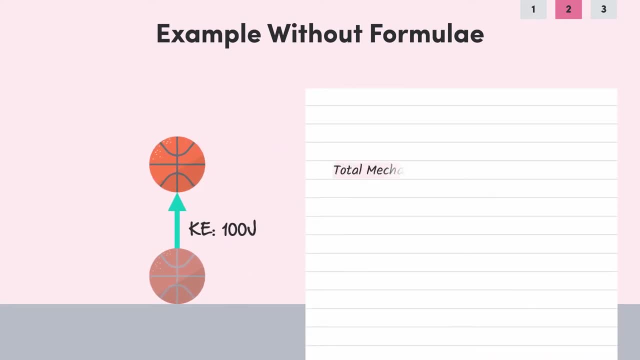 To apply energy conservation to the ball, we first need to calculate its total mechanical energy by adding the kinetic energy and the gravitational potential energy, The kinetic energy is given to us- it's 100 joules- but we still need the GPE, In this case the ball. 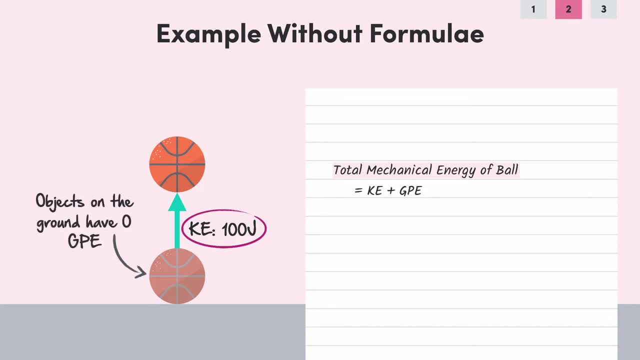 starts on the ground and we generally assume that objects on the ground have zero GPE. So we can say the total mechanical energy here is 100 joules of kinetic energy plus zero joules of GPE. This is 100 joules of kinetic energy plus zero joules of GPE, which is 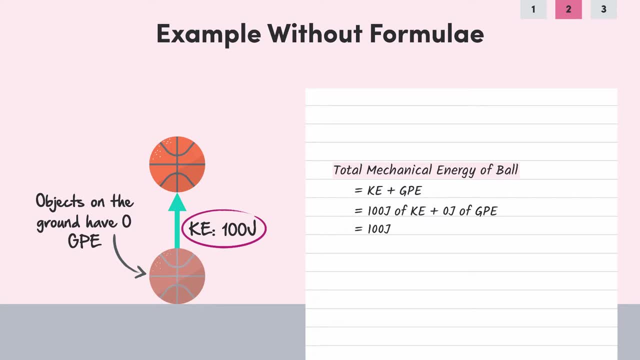 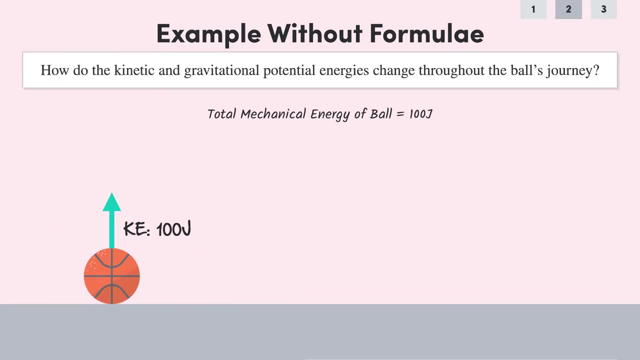 100 joules in total. Now, the most important thing to remember is that the total mechanical energy of the system never changes. It will always be 100 joules. That's what we mean when we say mechanical energy is conserved. So let's see how the kinetic and gravitational 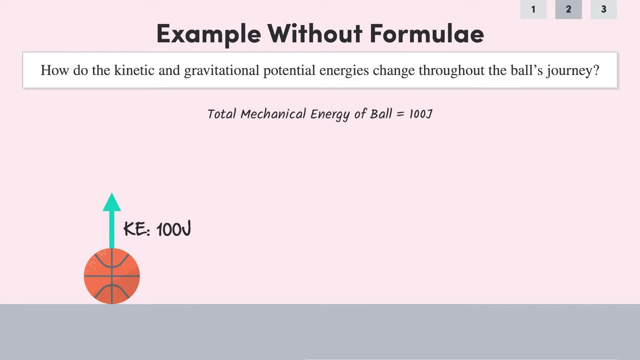 potential energy changes throughout the ball's journey. We'll assume that there's no air resistance involved here. So at the start the ball is at its fastest. This is because its kinetic energy is at a maximum. As the ball rises in height above the ground, it 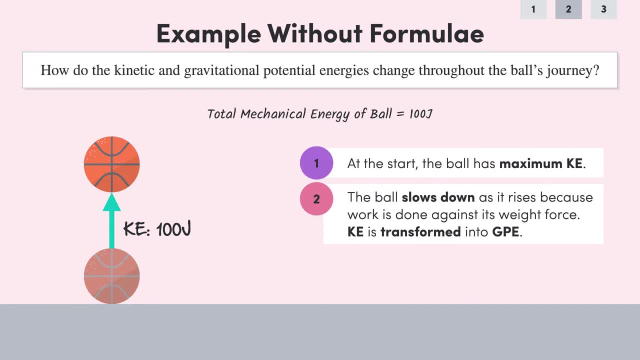 slows down as it does work against its weight force. As it slows and rises, its kinetic energy is transformed into gravitational potential energy. So if its kinetic energy is 50 joules, its GPE is also 50 joules, because KE plus PE always adds up to 100 joules. 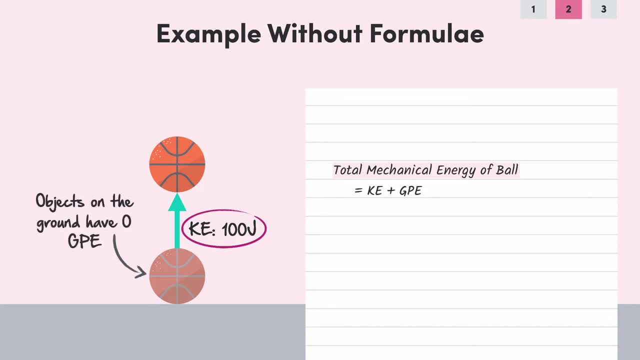 starts on the ground and we generally assume that objects on the ground have zero GPE. So we can say the total mechanical energy here is 100 joules of kinetic energy plus zero joules of GPE. This is 100 joules of kinetic energy plus zero joules of GPE, which is 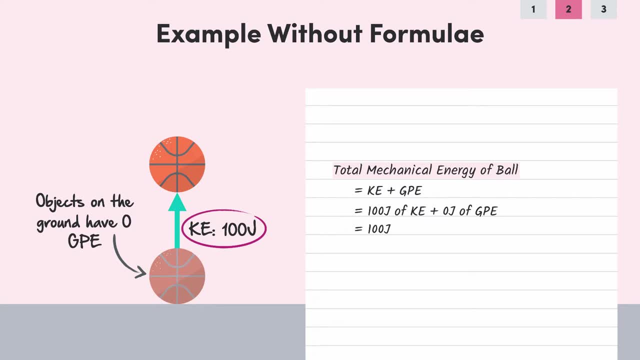 hundred joules in total. Now, the most important thing to remember is that the total mechanical energy of the system never changes. It will always be 100 joules. That's what we mean when we say mechanical energy is conserved. So let's. 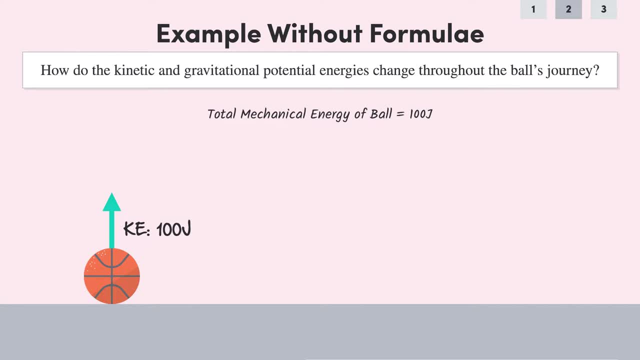 see how the kinetic and gravitational potential energy changes throughout the ball's journey. We'll assume that there's no air resistance involved here, So at the start the ball is at its fastest. This is because its kinetic energy is at a maximum. As the ball rises in height above the ground, it slows down as it. 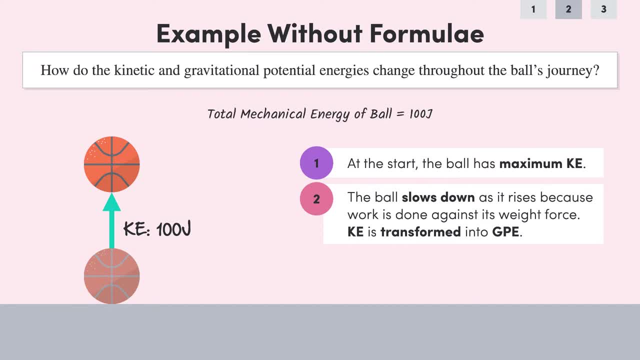 does work against its weight force. As it slows and rises, its kinetic energy is transformed into gravitational potential energy. So if its kinetic energy is 50 joules, its GPE is also 50 joules, because Ke plus Pe always adds up to 100 joules. 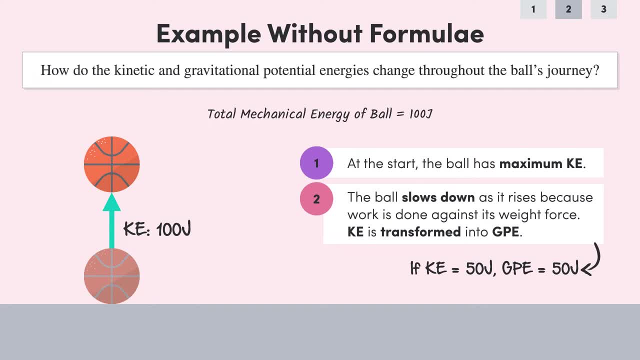 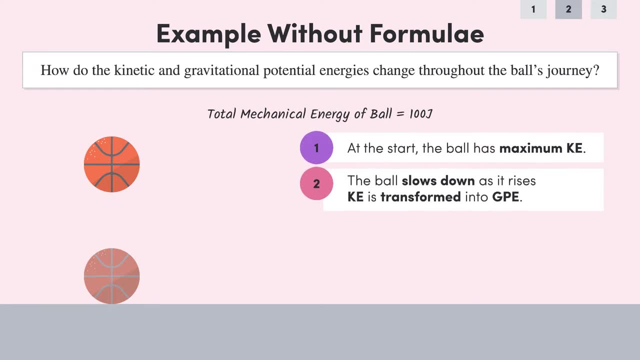 Notice here. we didn't even need a formula to calculate the GPE. We just need to use our knowledge about the conservation of energy. Okay, so now let's see what happens when the ball reaches its maximum height At the top of its flight. all the kinetic energy has been 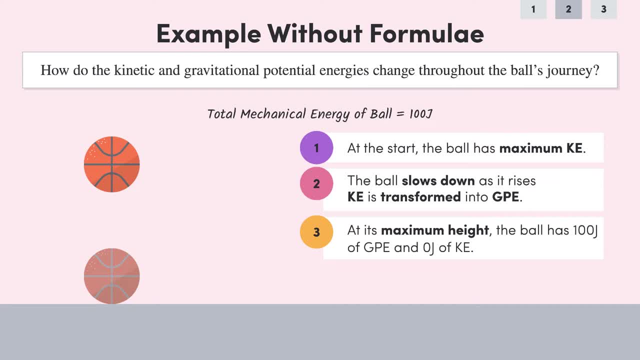 converted to GPE. So the GPE here has to be equal to 100 joules. Since the total mechanical energy is 100 joules, that means the kinetic energy must be zero joules. This tells us something important. At the top of the ball there's a 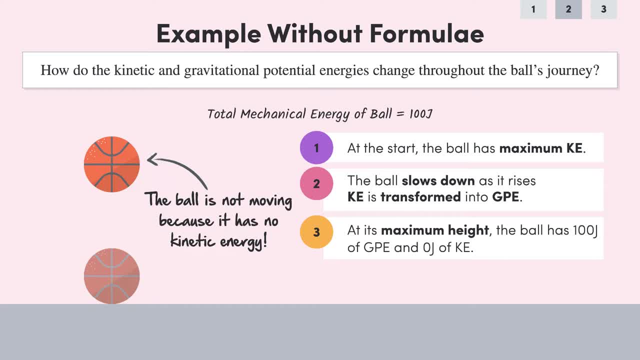 small amount of kinetic energy in the air. So when the ball is flying, the ball is not moving because it has zero kinetic energy. That might be a wacky idea to get your head around, but have a go at throwing some balls in the air and try. 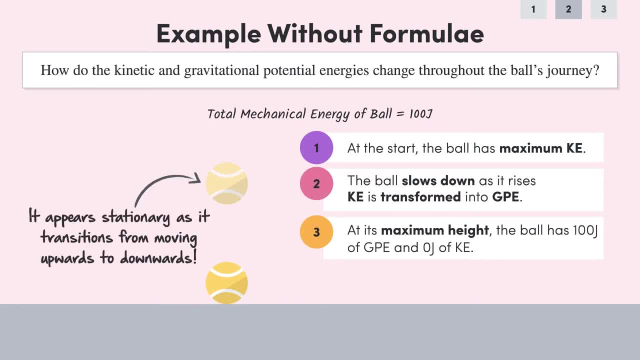 to pay close attention to the ball's velocity at the top of their flights. You'll see for a split second the ball looks as if it's stationary as it transitions from moving upwards to downwards. At this exact moment, all the kinetic energy has been converted to GPE. 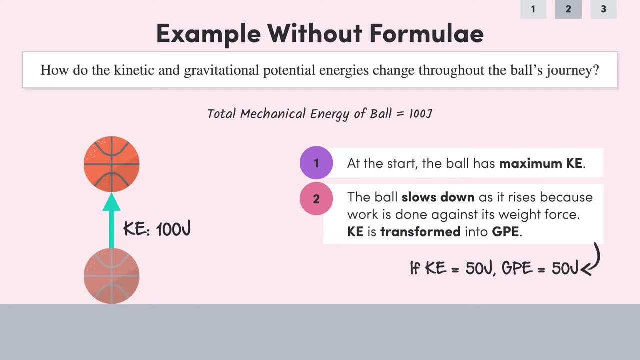 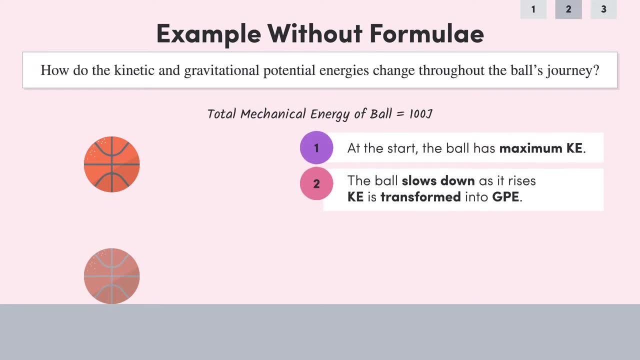 Notice here. we didn't even need a formula to calculate the GPE. we just need to use our knowledge about the conservation of energy. OK, so now let's see what happens when the ball reaches its maximum height At the top of its flight. all the kinetic energy has been converted to GPE, So the GPE here has 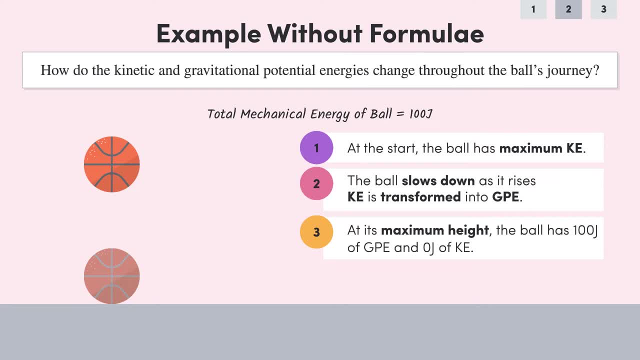 to be equal to 100 joules. Since the total mechanical energy is 100 joules, that means the kinetic energy must be 0 joules. This tells us something important. At the top of the ball's flight. the ball isn't moving because it has 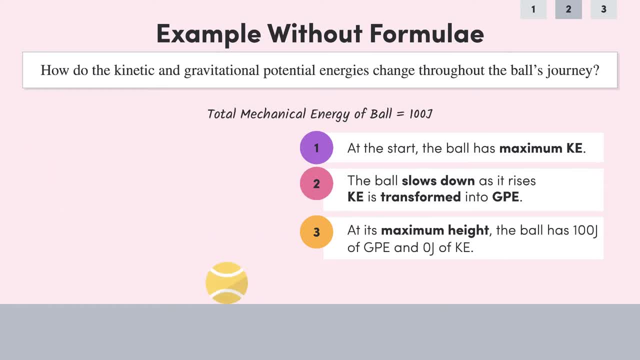 zero kinetic energy. That might be a wacky idea to get your head around, but have a go at throwing some balls in the air and try to pay close attention to the ball's velocity at the top of their flights. You'll see for a split second. the ball looks as if it's stationary as it transitions. 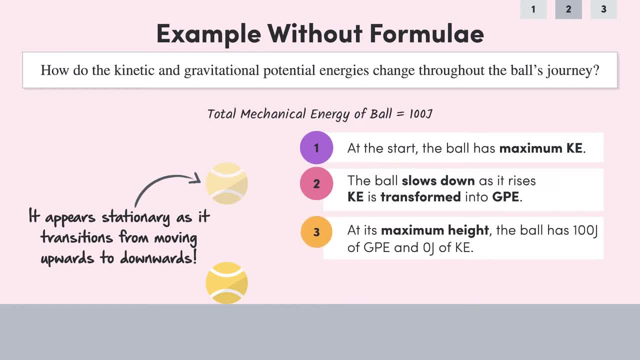 from moving upwards to downwards. At this exact moment, all the kinetic energy has been converted to GPE. And last off, let's analyse what happens when the ball travels back towards the ground. The GPE is gradually converted back to kinetic energy, so the ball speeds up as it falls towards. 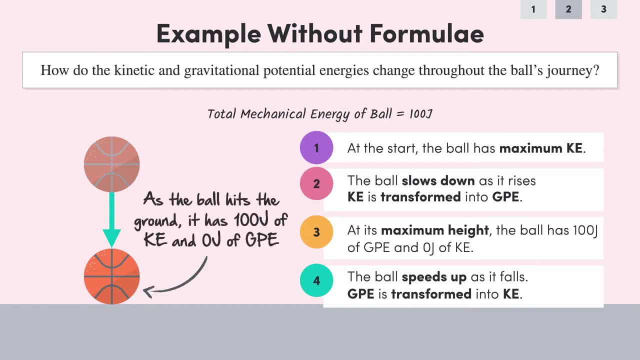 the ground. At the precise moment the ball reaches the ground, it once again has 100 Joules of kinetic energy and 0 Joules of GPE. The key takeaway here is that, no matter what part of the journey we're on- beginning, middle or end- the total mechanical energy is always constant. 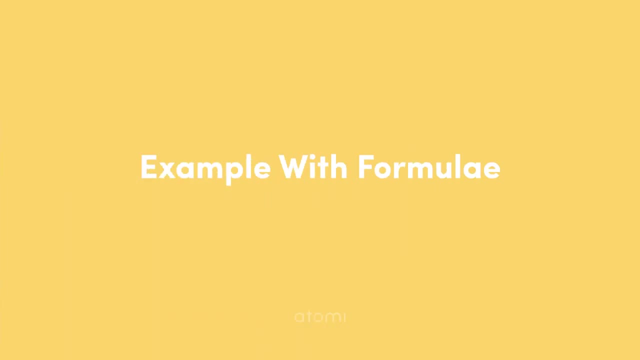 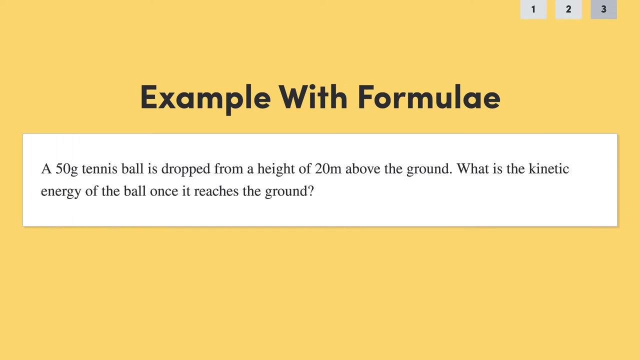 Okay, so let's do a quick example of a question you might get asked in the comments section of this video: What is the kinetic energy of a ball? What is the kinetic energy of a ball that involves our energy formulae? Let's say you drop a 50 gram tennis ball from a height of 20 metres above the ground. 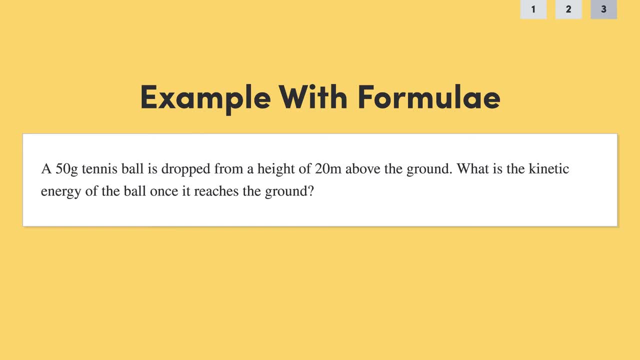 What is the kinetic energy of the ball once it reaches the ground? At first glance, it looks like we can't calculate the kinetic energy because we aren't given the ball's velocity, and so we can't use the equation. KE equals a half mv squared. 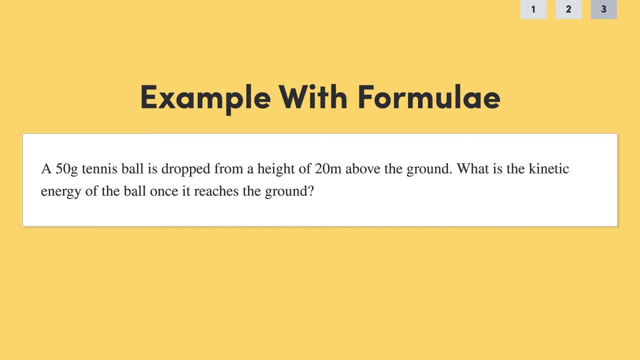 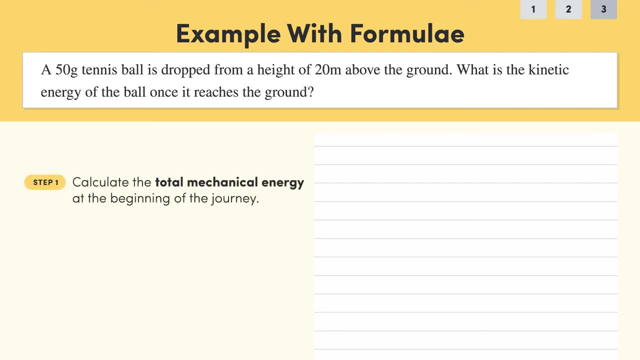 But luckily for us, we know a thing or two about the conservation of mechanical energy. So the method for solving this problem is to first calculate the total mechanical energy at the beginning of the journey and then use the conservation of mechanical energy to find the 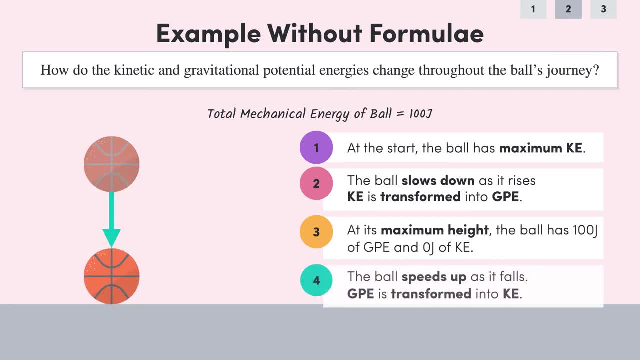 This happens when the ball travels back towards the ground. The GPE is gradually converted back to kinetic energy, So the ball speeds up as it falls towards the ground. At the precise moment the ball reaches the ground, it once again has 100 joules of kinetic energy and zero joules of GPE. The key takeaway here is: 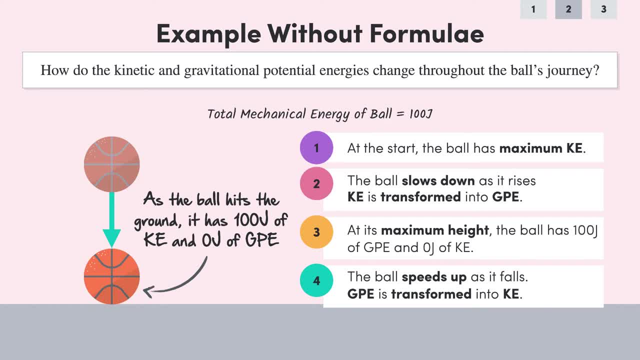 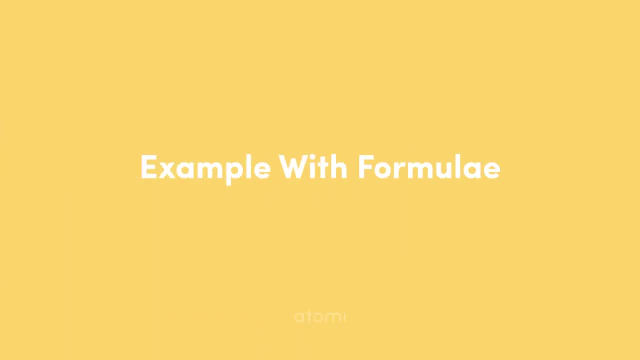 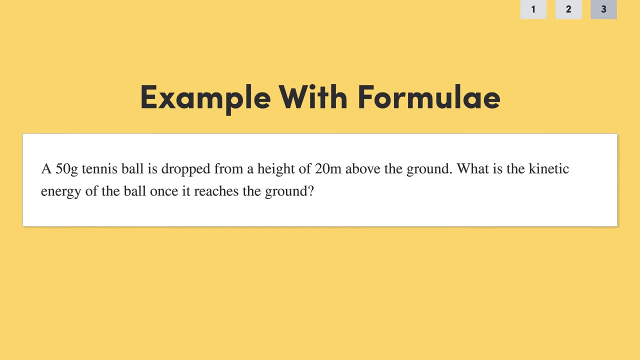 that no matter what part of the journey we're on- beginning, middle or end- the total mechanical energy is always constant. Okay, so let's do a quick example of a question you might get asked in your exams that involves our energy formulae. Let's say you drop a 50 gram tennis. 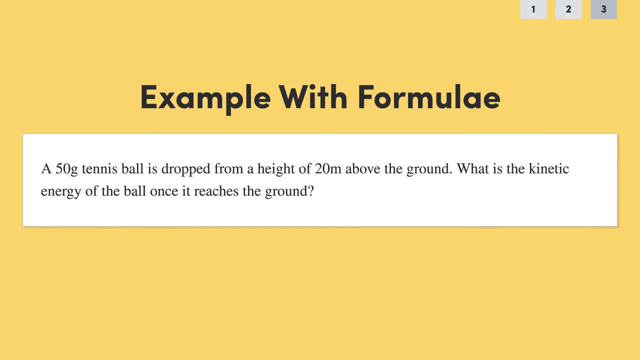 ball from a height of 20 meters above the ground. What is the kinetic energy of the ball once it reaches the ground? At first glance, it looks like we can't calculate the kinetic energy because we aren't given the ball's velocity, and so 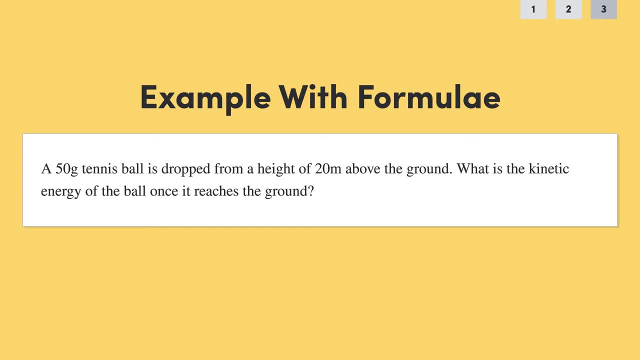 we can't use the equation ke equals 1⁄2 mv squared. But luckily for us we know a thing or two about the conservation of mechanical energy. So let's start energy. So the method for solving this problem is to first calculate the total mechanical energy. 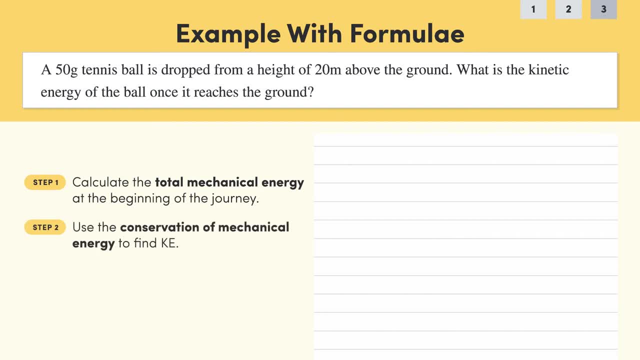 at the beginning of the journey and then use the conservation of mechanical energy to find the kinetic energy at the end of the journey. It's as simple as that At the beginning of the journey, just as we drop it, the ball is stationary, so its kinetic energy is zero joules. 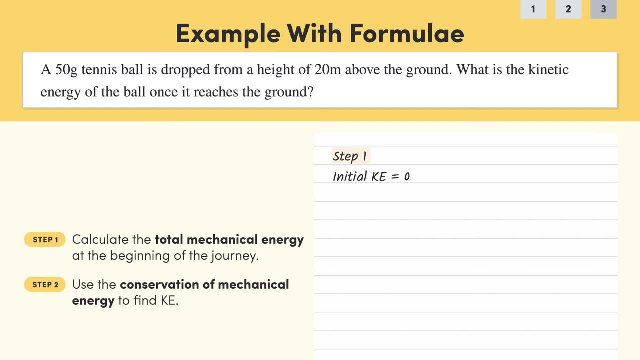 We can calculate the GPE using our trusty formula: GPE equals mgh. Be careful with the units here. We first need to convert from grams to kilograms. 50 grams equals 0.05 kilograms. We know g: the Earth's gravitational acceleration is 9.81 m per second squared. 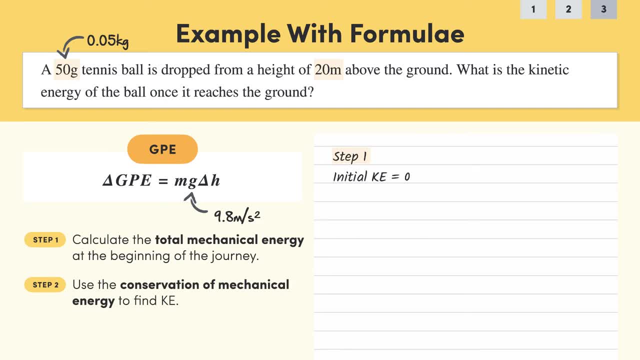 and the height is the height above ground, 20 meters. That means we can say GPE equals mgh, which equals 0.05.. 0.05 x 9.81 x 20,, which equals 9.81 Joules. This is the amount of GPE the object has. 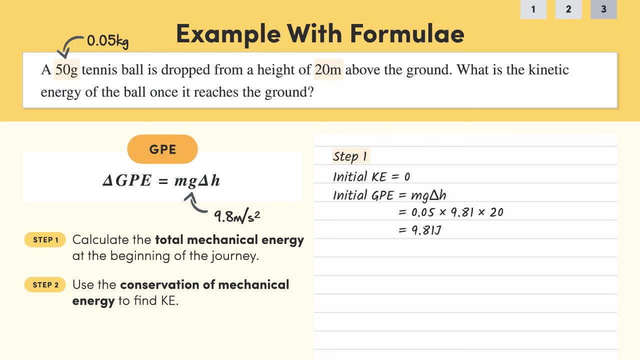 due to it being lifted 20 metres off the ground. So the total mechanical energy is Ke plus GPE- equals 0 Joules plus 9.81 Joules, which equals 9.81 Joules, And we are actually pretty much finished once we have this. 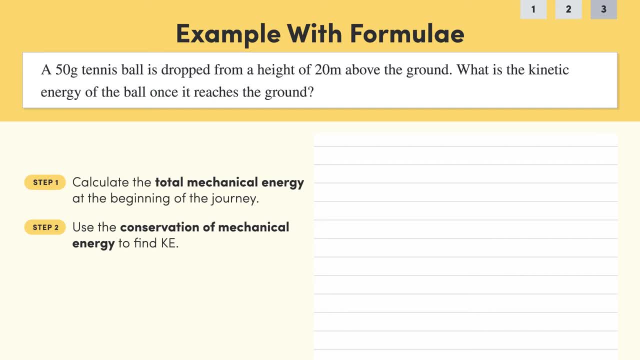 kinetic energy at the end of the journey. It's as simple as that. At the beginning of the journey, just as we drop it, the ball is stationary, so its kinetic energy is 0 Joules. We can calculate the GPE using our trusty formula: GPE equals mgh. Be careful with the units here We 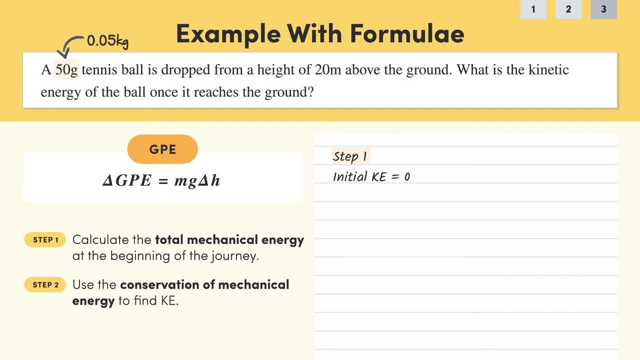 first need to convert from ground to ground and then we need to convert from ground to ground. So GPE equals mgh, We know G. the Earth's gravitational acceleration is 9.81 metres per second squared and the height is the height above ground: 20 metres. 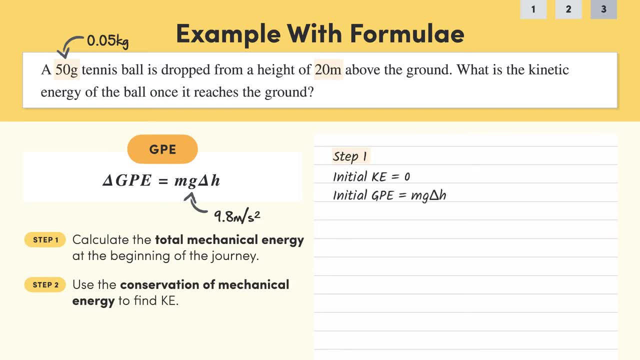 That means we can say: GPE equals mgh, which equals 0.05 times 9.81 times 20,, which equals 9.81 Joules. This is the amount of GPE the object has due to it being lifted 20 metres off the ground. So the total mechanical energy is KE. 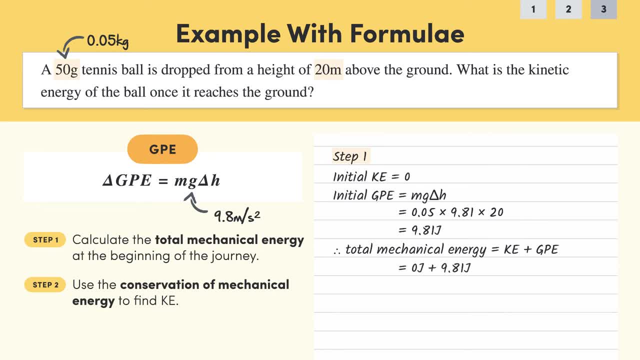 plus GPE equals 0 Joules plus 9.81 Joules, which equals 9.81 Joules, And we are pretty much finished once we have this. Since the total mechanical energy is always conserved, that means that at the end of 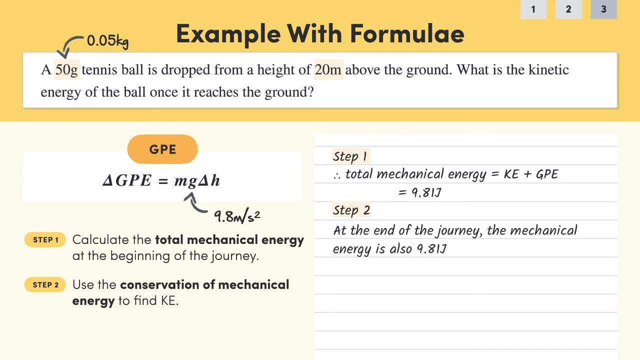 the journey. the mechanical energy is also 9.81 Joules. When the ball reaches the ground, its GPE zero joules, so its kinetic energy has to be the full 9.81 joules And that's it OK. so just a little tip. we could also use this result to calculate the velocity of the ball. 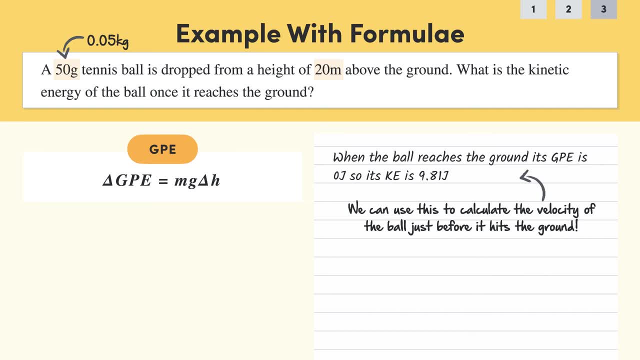 just before it hits the ground. To do this we would rearrange the kinetic energy equation to make velocity the subject. Ke equals a half mv squared. 9.81 equals 0.5 times 0.05 times v squared. So v squared equals 9.81 over 0.025.. Therefore v equals 19.8 m per second. How cool. 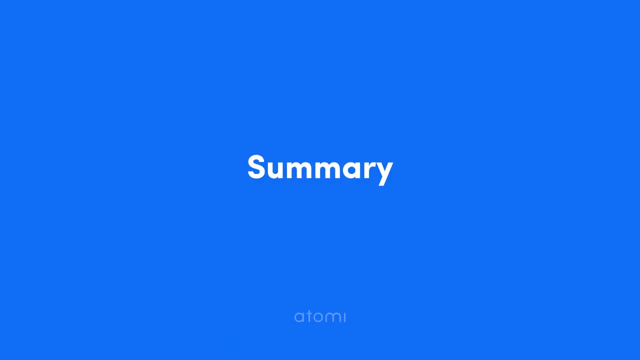 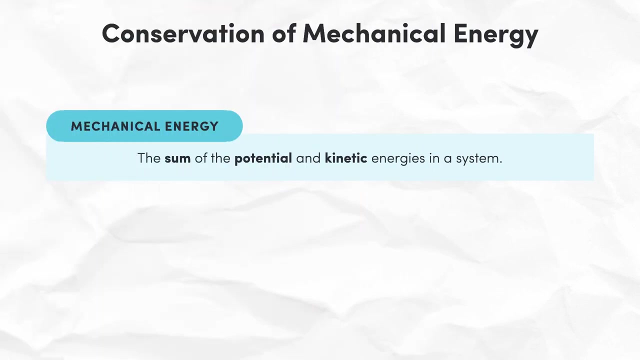 is that, And there we go. That's all we have for this content, so let's summarise. We started off by defining mechanical energy as the sum of the kinetic energy and potential energy in a system. The most important thing you need to remember from.